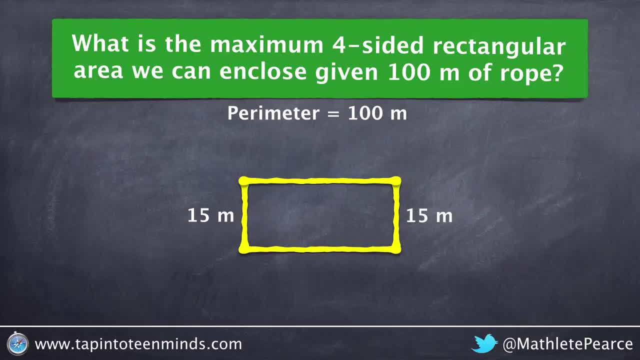 Since we have two lengths, we'll divide that 70 meters by 2, and we'll end up with 35 meters for both of our lengths. Calculating the area of this rectangle will have us multiply the length of 35 meters by the width of 15 meters, yielding a total area of 525 meters squared Again. 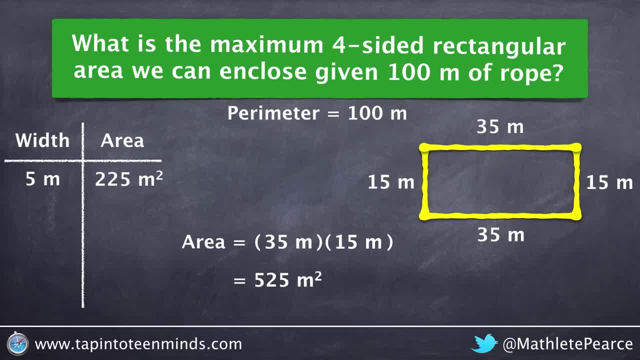 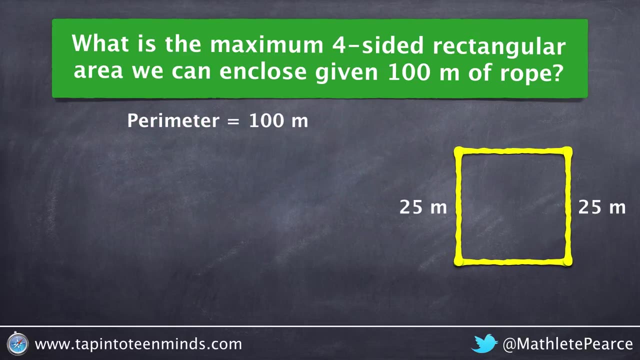 taking a look at the relationship between the width and the area, and we have a width of 15 meters and our area will increase to 525 meters squared. Investigating further, we could increase our width to 25 meters, for example, which would yield 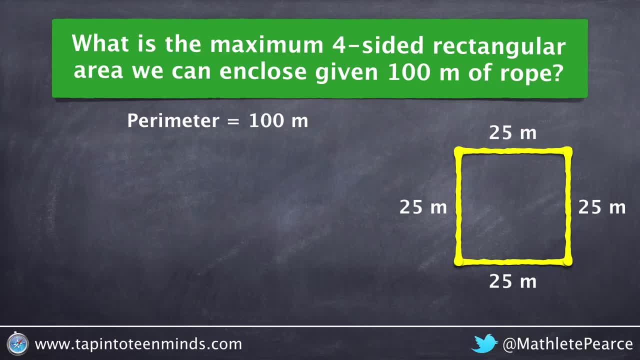 a square. We would have two widths of 25 and two lengths of 25 to use the entire 100 meters of rope. Calculating the area of this special rectangle or square, we would multiply the length of 25 meters by the width of 25 meters, for a total area of 625 meters squared. Going back to our 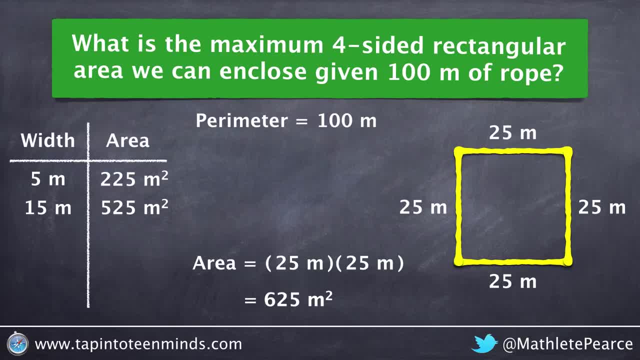 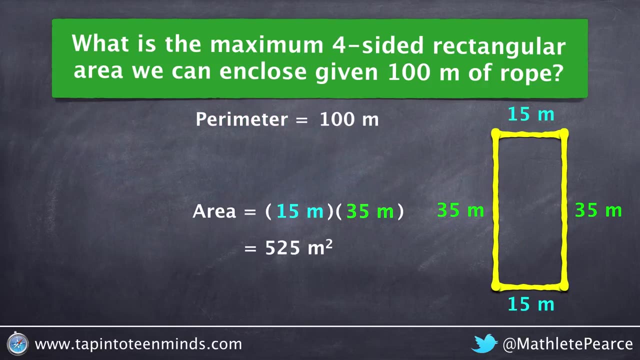 relationship between width and area. we can see that when the width is 25 meters, our area has increased again to 625 meters squared. Continuing our exploration, we're going to increase the width to 35 meters, which will leave us with 15 meters for our lengths And when we look at our table. 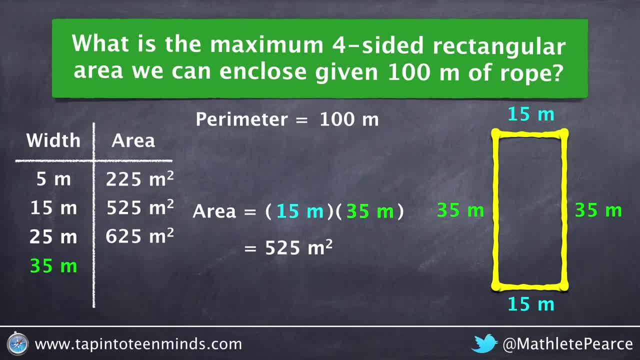 we'll notice that when the width was 15 meters, the length was 35 meters. Now our width is 35 meters and our length is 15 meters, So essentially we're going to get that same area of 525 meters squared Again. if we look at the width of 45 meters, for example. that's going to leave us. 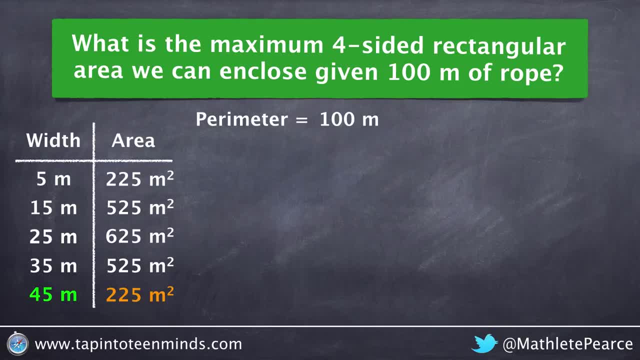 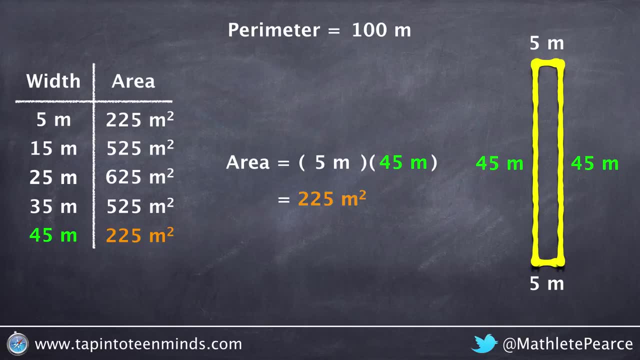 with only a length of 5 meters, giving us again an area that we've already seen before at 225 meters squared, And essentially all we're doing here is taking the rectangle from being narrow horizontally to a really narrow and vertical rectangle. So, in conclusion,